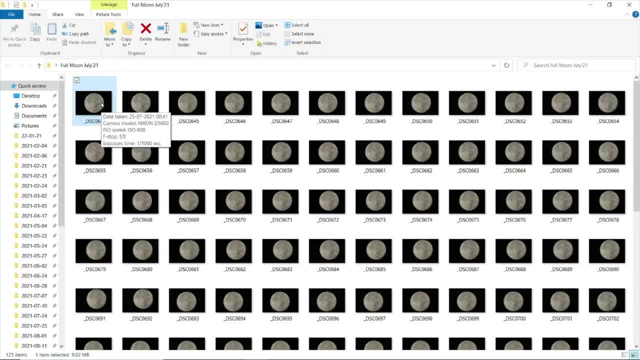 you would like to keep the ISO down to, let's say, 100.. But in full moon's case, what I have learned from few of the other astro imagers that it's always better to increase your ISO, at the same time increase the shutter speed. 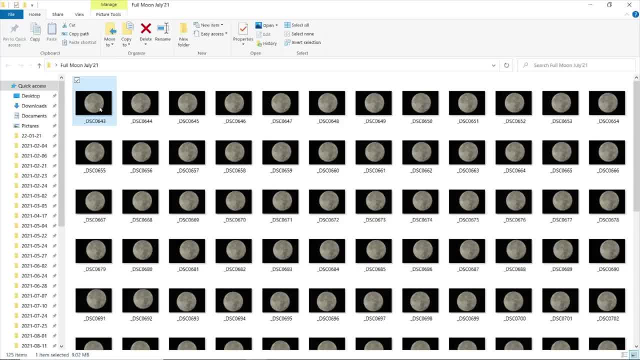 So what? my advice would be to look at your histogram, because histogram never lies. It's your friend. Look at the histogram and ensure that it is speaking in the middle. It's not at the far left. It's not at the far right. 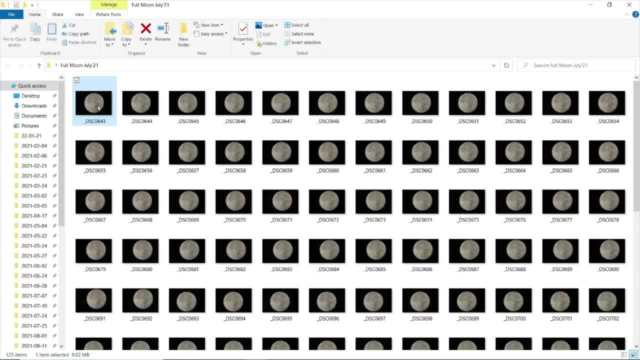 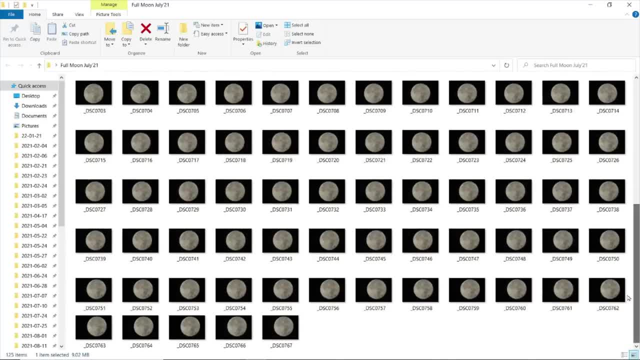 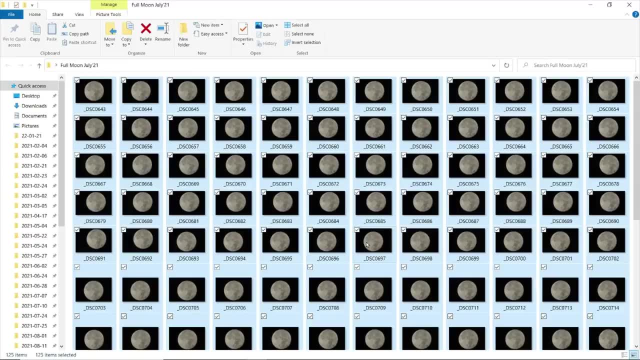 So it makes your processing very easy. Now these are about 125 images that I've taken. That's the count that I'm getting. I would not recommend such a large cache of files, but I do take normally more than 100 because sometimes my tracking 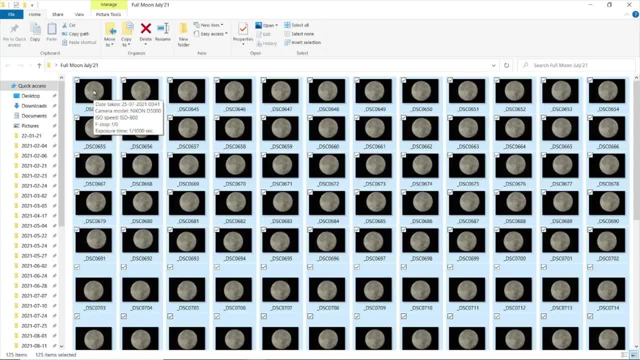 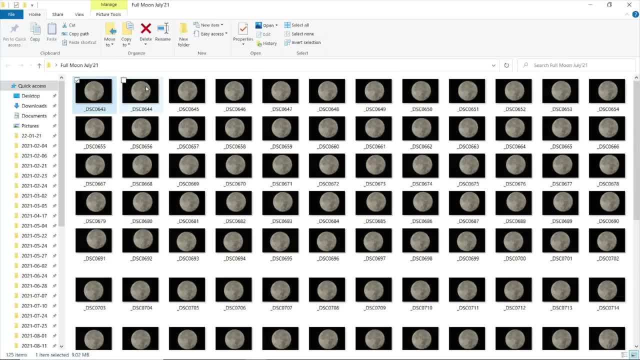 I'm not tracking on equatorial mount, I'm tracking on an equatorial platform, So the images tend to, you know, waver a bit. I can cut on one part of the object and then you know, the whole set is ruined. 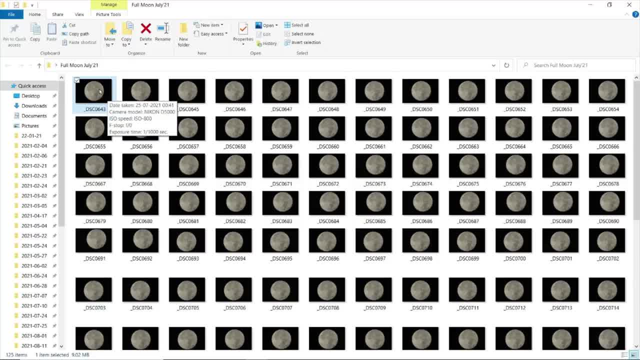 So I, as a precautionary measure, I do take more than 100.. But even if you have 30, 40 images, the result is going to be good, It's not going to be bad. So this is the data of the raw images that I have. 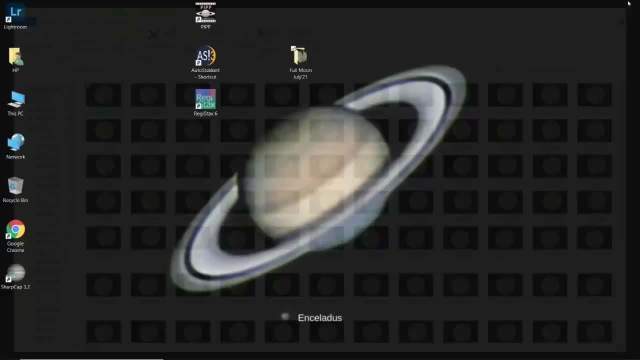 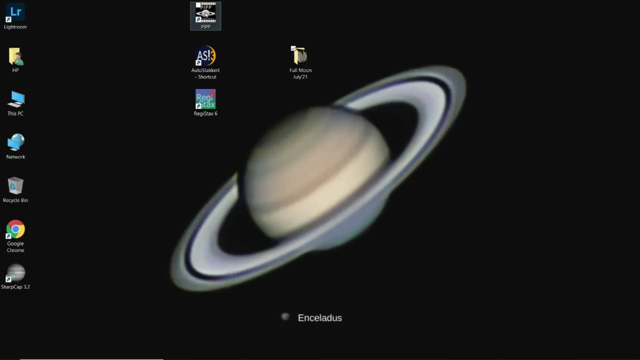 that I've just opened. So let's jump into the process. We are going to be using our three friends- You know this from my previous tutorial- the free softwares, pip order stacker and register stacks. The same process applies here. 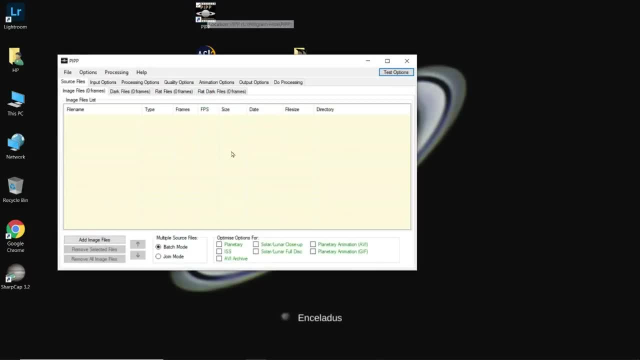 We will start with pip because we have shortened manual mode and we have NEF file. We need to take it to order stacker. So we are going to use pip and we're going to center the object because there was a little shift in each batch that I shot. 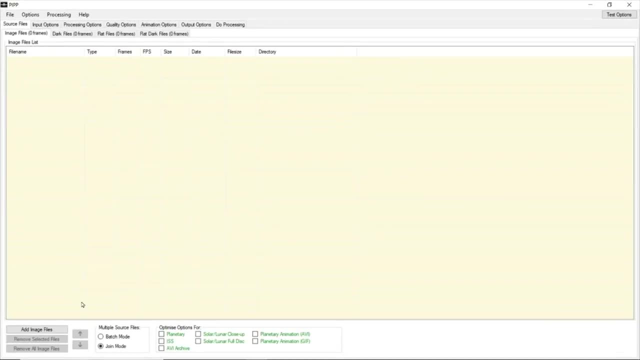 So take a look at this This. you have to ensure that you are using join mode because it's individual raw file and you're going to click on solar lunar full disk. That's all we need to do. We can add images from here or we can open file. 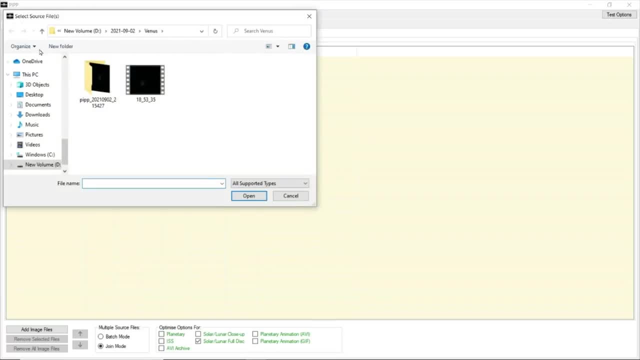 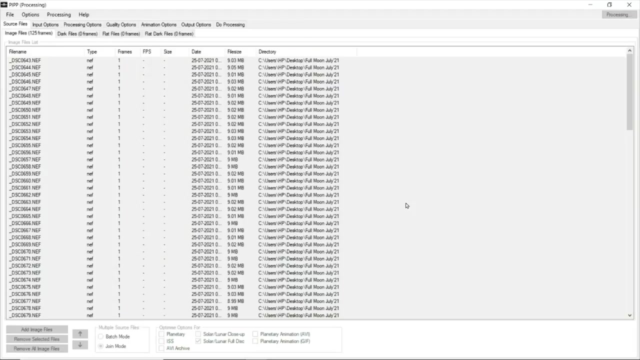 We can add source from here. There are many ways of doing this. This is the folder that I have created on the desktop with all the data of 125 single images that I've taken. So this is how the data look. Ignore this. 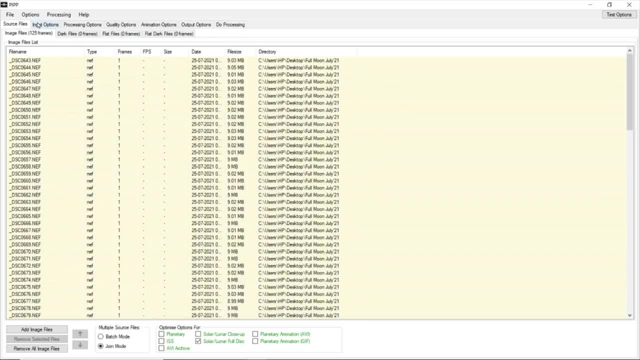 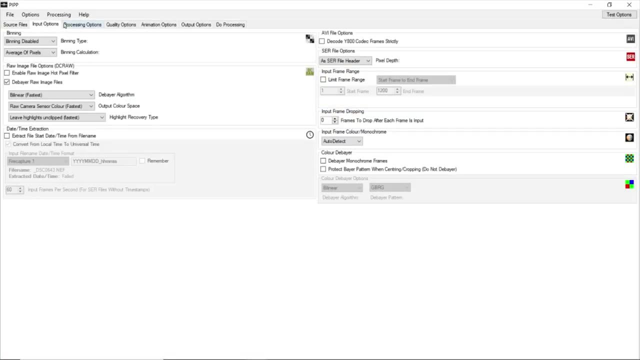 We're going to take a look at this Now. the most important part is you've added in the source file. Input is something that you don't have to do anything. You don't have to do anything here, Just leave it at default. 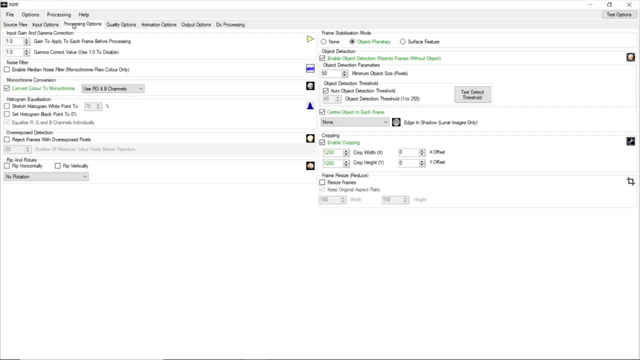 Processing options is very important. Now, this is something which is a critical step. First of all, you'll see that convert color to monochrome is automatically ticked. Ensure that you uncheck this. You don't want a monochrome color. You don't want a gray scale picture. 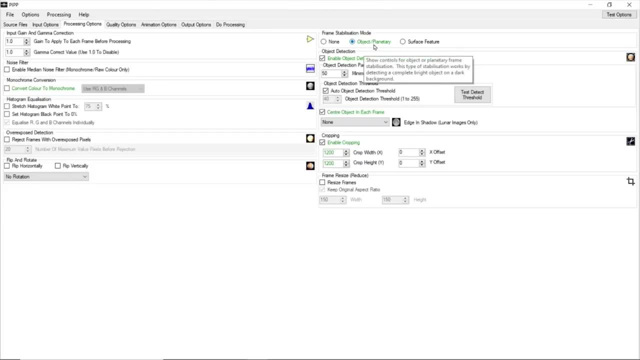 This is one. Second is object should be planetary. It's a spherical disk, So that's what you have to do, But you have to ensure that it's clicked on this Enable object detection. Yeah, fair, Because if sometimes you know, 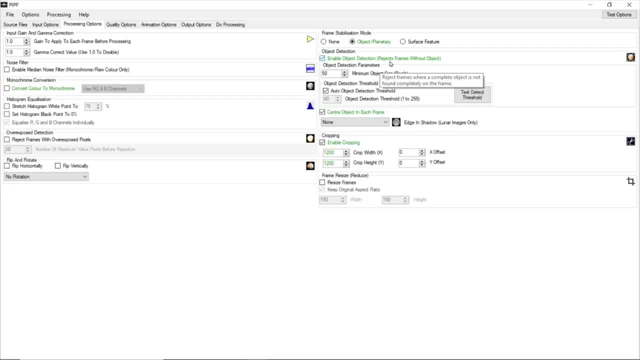 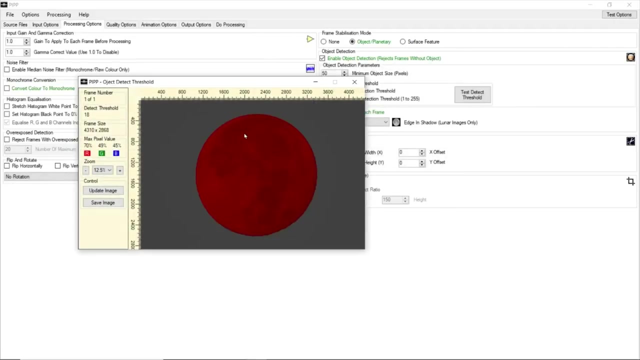 the tracking goes haywire and the object tends to touch the edge of the frame, then it's better not to have that. This is fine And we can test the detect threshold. It's showing you full moon Now. it's very important for you to understand that when you're shooting full moon at 1200mm, 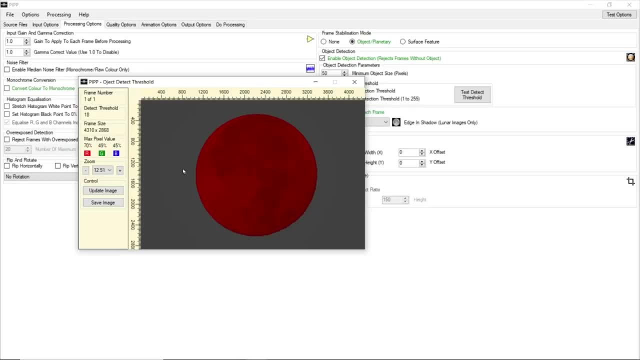 and you're using a telescope instead of a lens. with a DSLR, you tend to get a lot of black space around, And that is just going to help you with nothing. It's just going to increase the file size. So just ensure you do a bit of cropping. 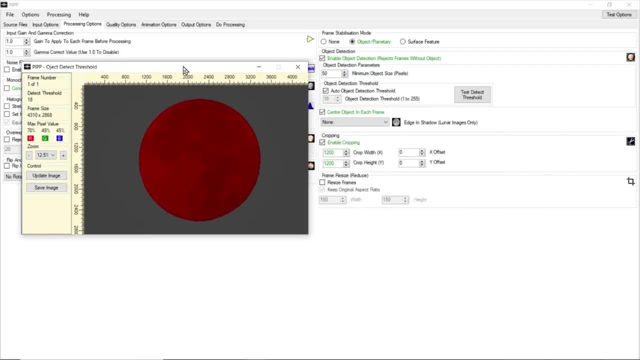 Now, if you look by default, the cropping is coming at 1200 by 1200.. If we do 1200 by 1200, by the scale, I don't think we're going to get the full disc of moon. 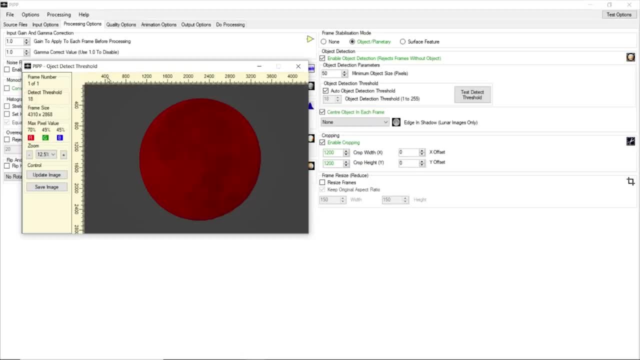 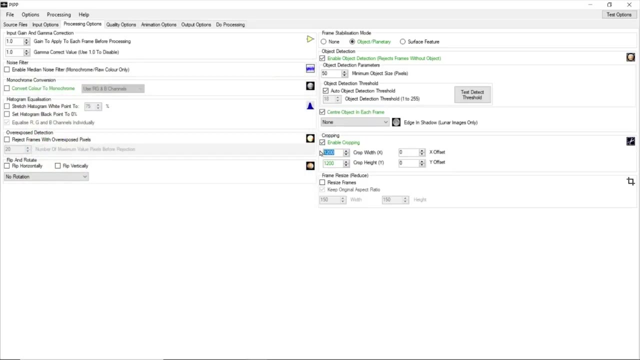 So, just you know, by checking the scale here and both the axes, you can ensure the crop area that you take is quite feasible to your image. So what I normally do is I keep it at 2800 by 2800. So that's it. 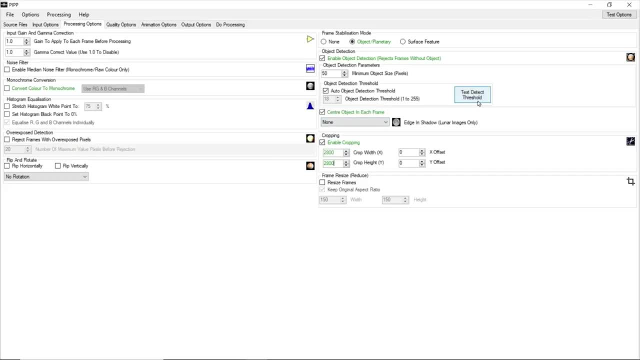 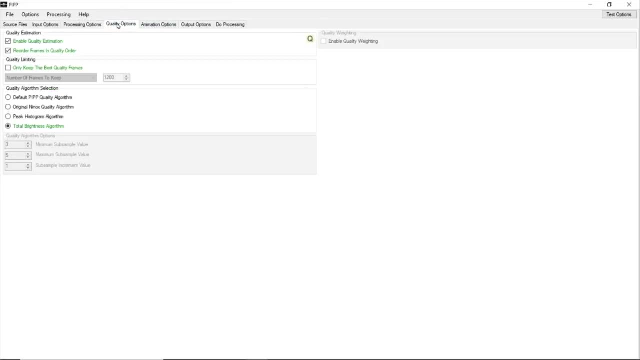 So that's where I can see that my whole image comes into the frame. We don't have to work about the quality options. We are not animating output. We're going to ensure that it is in TIFF format. That will help you. 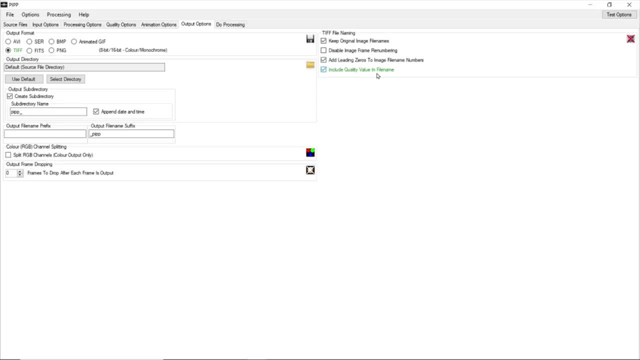 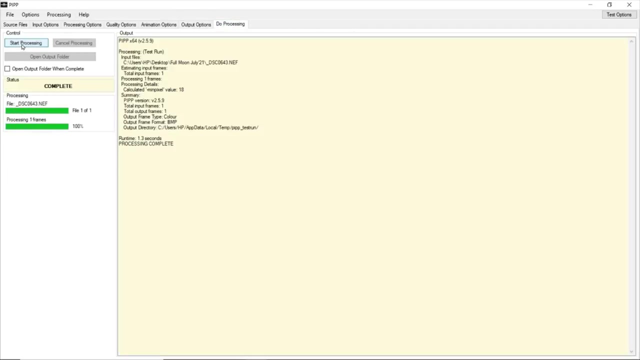 And just ensure that include quality value and file name is ticked. It's going to show you the brightness of your frames, which will going to help you in deciding what data to use in further stacking. Let's click on do processing. Very simple process. 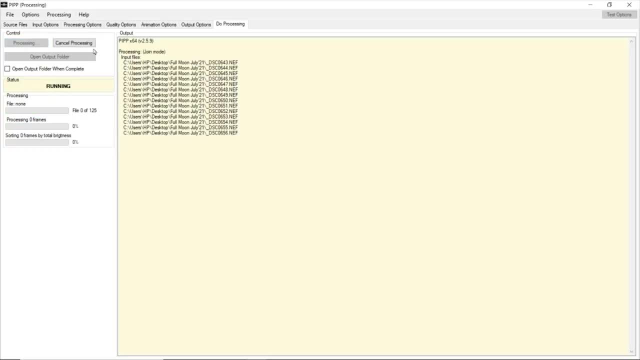 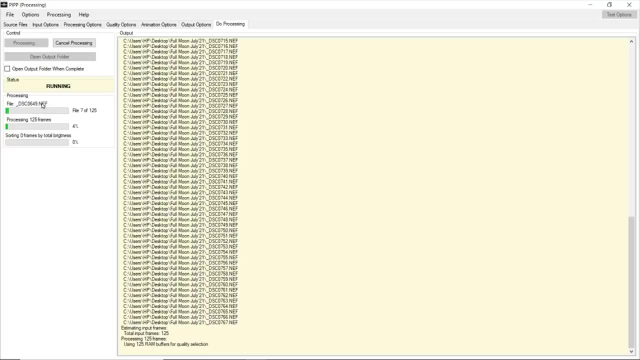 Again, we have just to press start processing and you would see that it's just not processing your raw files into TIFF file. It is also going to sort your frames by total brightness. You know, in the last step this is exactly going to do the sorting of the frames according to the brightness. 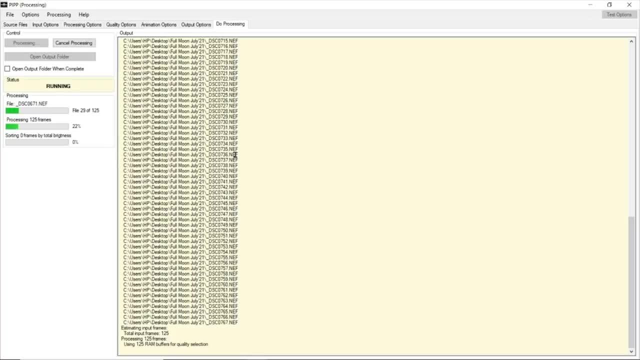 And in case, when you further process it, if you feel that it's going below, let's say even 80%, then you can, you know, automatically delete that data. You don't want that A fairly simple process in PIP. 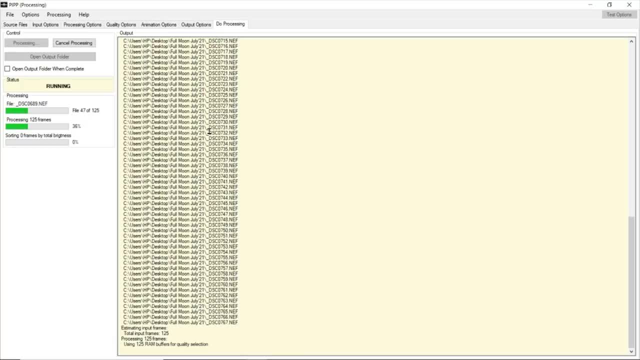 but it is essential. It gives you a lot of insight into what you have captured And it helps the process. So I'll take a pause here. I'll come back to you once this whole process is sorted. The process is complete. PIP has done its task. 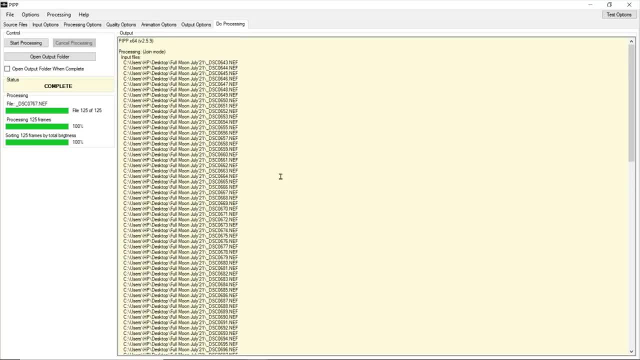 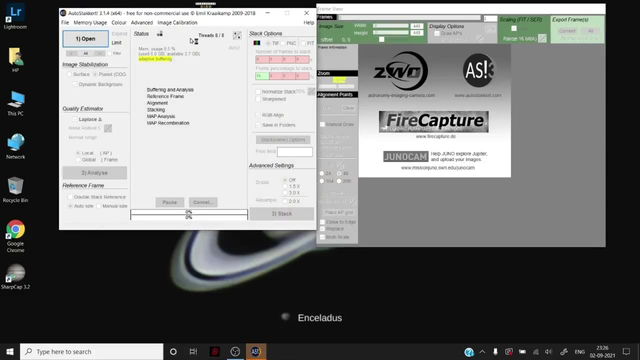 It has stabilized your object into the frame. It has sorted the frames through total brightness. So let's go to our next stop, which is going to be AutoStackered. And again, AutoStackered is going to be fairly simple in this process. 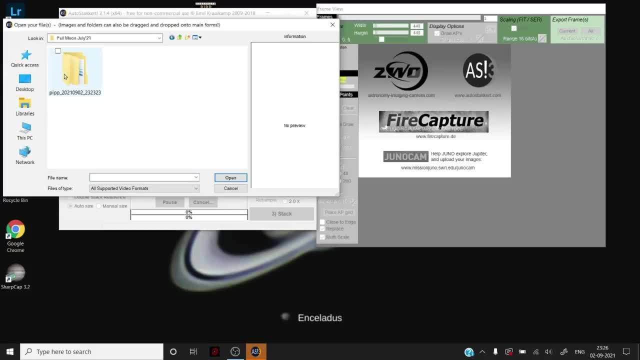 There is not going to be anything different than we did for the. Now you would see that by default it opens to all supported video formats and you would not find this because we have just processed in PIP and the output we chose as TIFF. 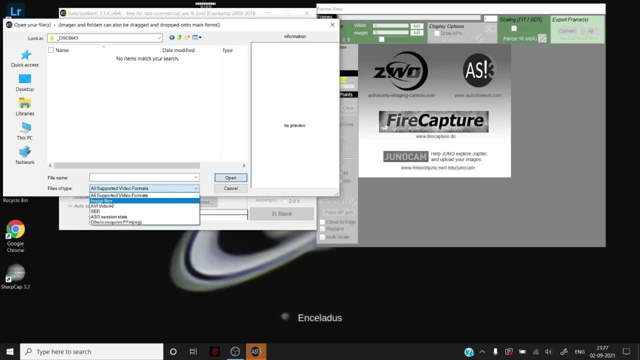 So it's not a video format. We just need to drop down the menu, ensure that we select image files and back. This is where you would see your data that you have processed in PIP. Now, as I said, it's going to do it quality-wise. 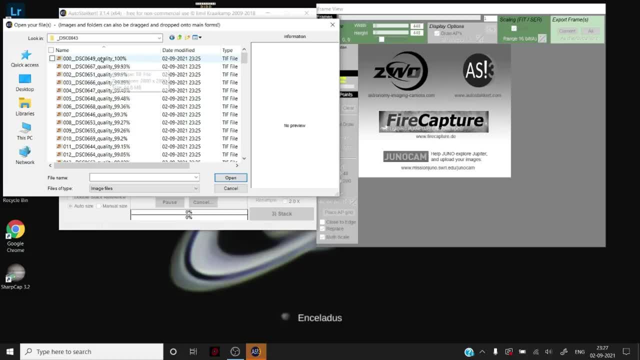 the brightness of the frames. If you look, this is how it has sorted. This is the PIP's interface, This is the PIP's data And this is the PIP's data that I have put. So almost all the files that has been put through: 94.52% is the last. 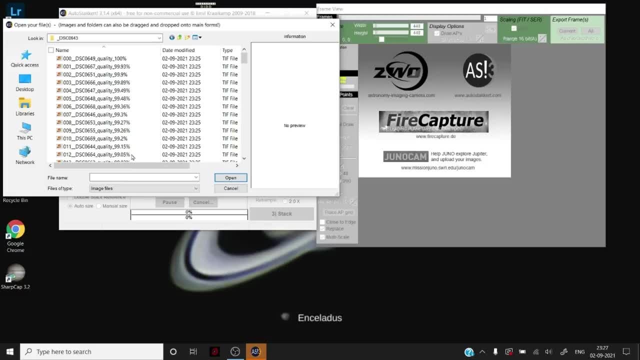 And I think that's a fair enough. That's a good amount of data that I have. I don't think that I need to delete anything. So I'm going to put everything in stacking, I'm going to select all the files And here we go. 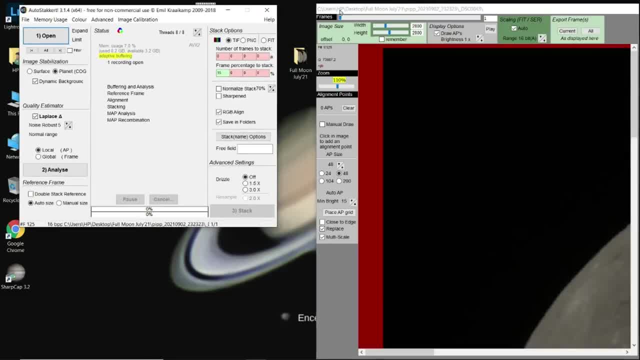 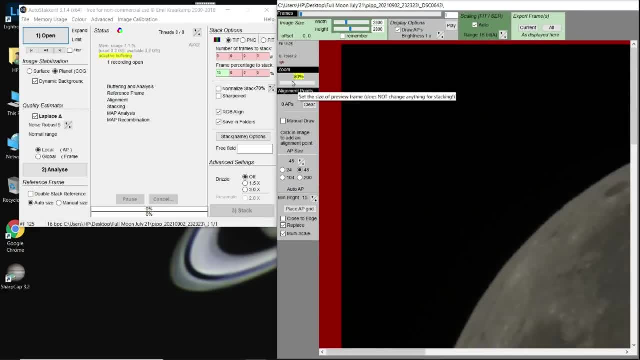 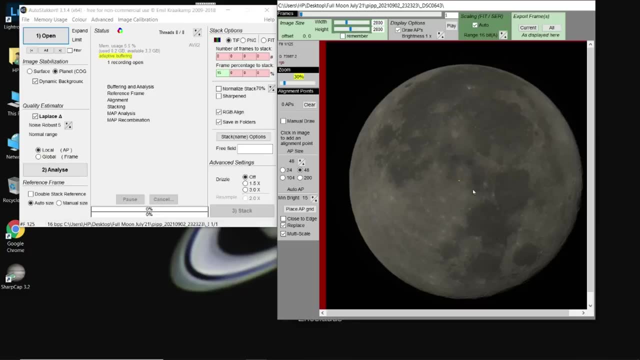 Now, this is normally. this is going to happen because, by default, the zoom proportion is quite big And, if you see, the size of the moon is quite big. So what we can do is we can easily put it at 20, 30% so that we can see the frame that is available to us. 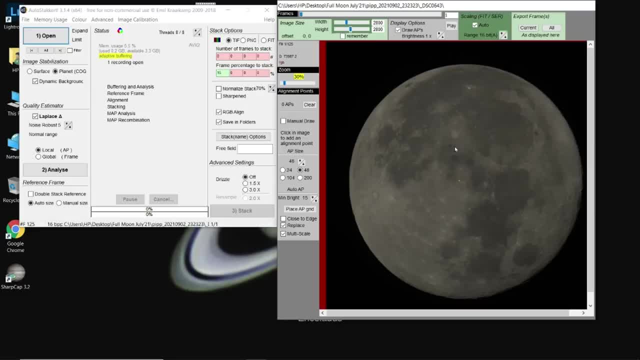 And remember that we cropped it, So it has come out, you know, quite neatly, but I see you know a balance of space. but we can always at the last step when we do something in Lightroom or Snapseed, 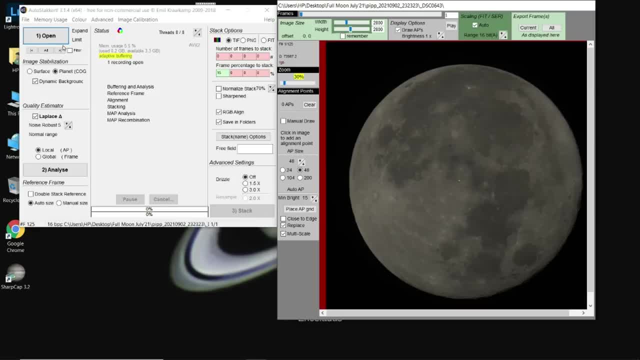 we can kind of rectify this. Now. let's go to this. We have opened, we have opened the PIP folder here. We have kept everything at default. We have chosen planet and let's do analyze. We know that the brightness is good. 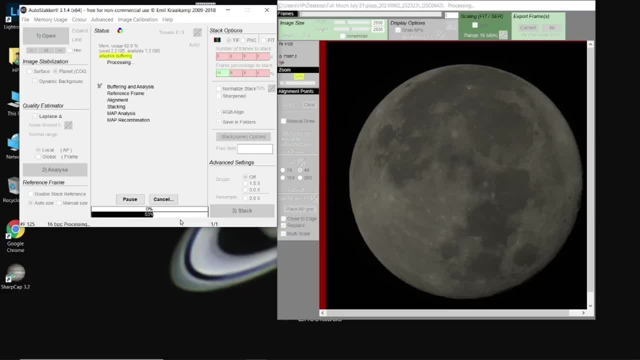 The last file was 94.5%, But let order stacker also give you an idea as to what it thinks of the quality of frames that you've put in. Okay, So my quality graph is: it's going down considerably after the midpoint. 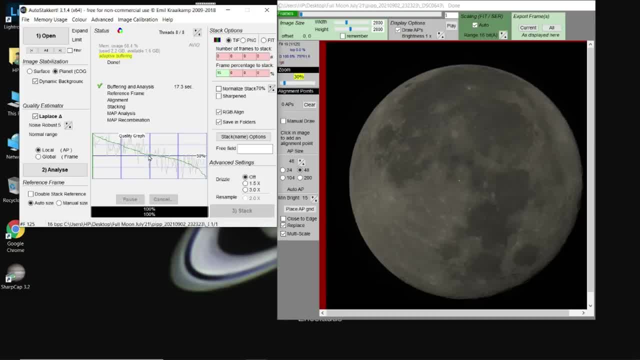 which is around 50%. It's a very simple press control and click here. So about 49, 50% of data we're going to use. So out of 125 frames, we're going to use 50% of this. 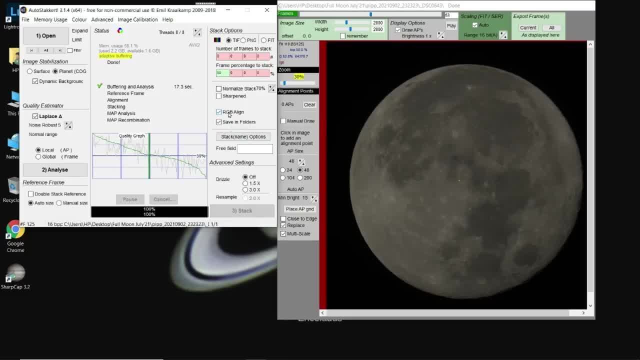 You can select RGB align. That's fair enough. Sharpened you're going to do in register stack. So again, I would not recommend to choose sharpened here. This is: this is something which is very standard, which we have already done in the last tutorial. 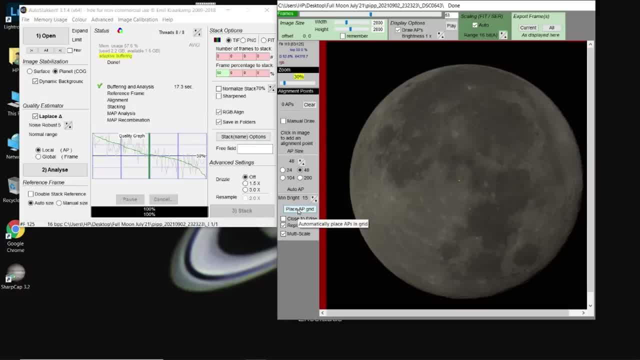 So let everything else remain default. We are going to place the the AP grid Now in AP grid. it's such a large object I would not recommend to use 4804.. Let's put the biggest alignment point size here And then just press AP grid. 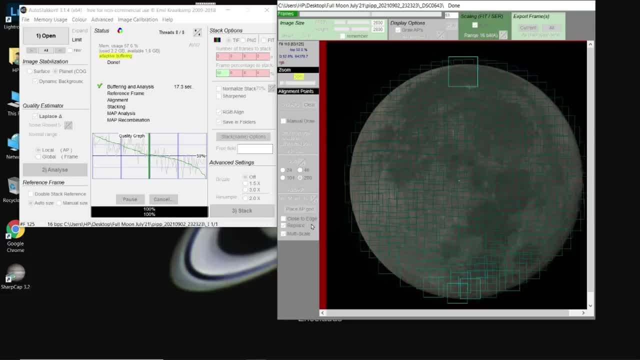 The alignment points are going to be placed automatically And we are done As we work along. or a stacker for any of my new audiences or new members who haven't seen any processes throughout a stacker. It is quite simple. Every tab gets activated. 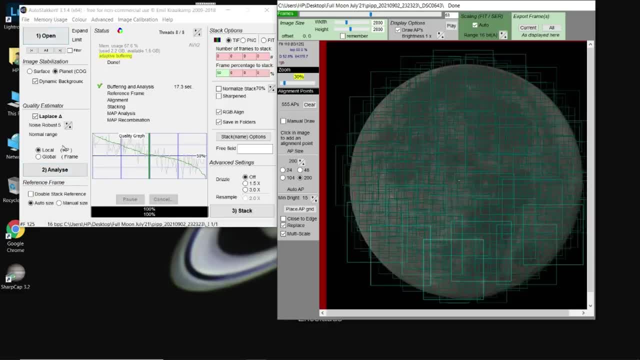 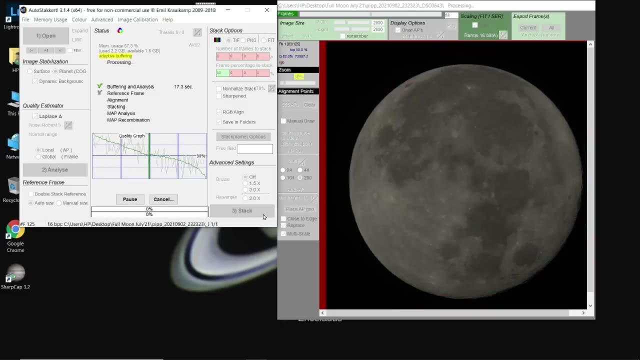 Once you finish the first one, the second will one will get activated. Now you see, the third option of stack is activated. So we are finished with the right hand side window. We are going to just press stack And it's going to take some time. 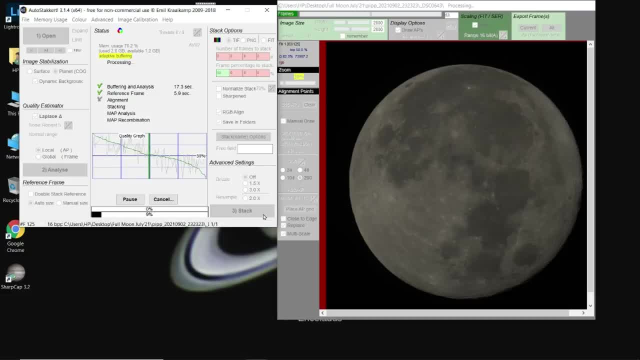 It's kind of fast, but yeah, it's going to take a while, And then we will take this stacked image. If you see one raw image, how dull and you know you don't see much details. but once we are through the stacking process, 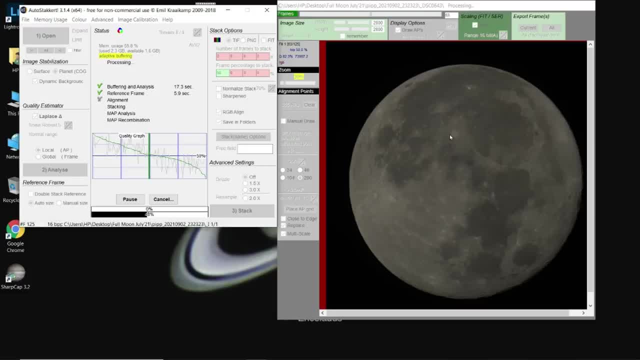 once we sharpen it and register stacks, you would see the transformation Your image will. you know the appearance of the image will make. Okay, So alignment, we are at alignment. Then it's going to do stacking. So let me pause here and let me come back. 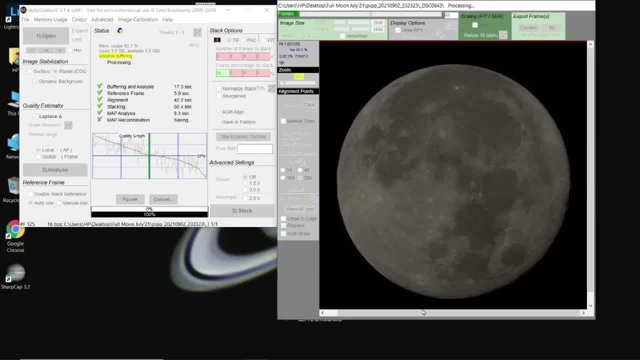 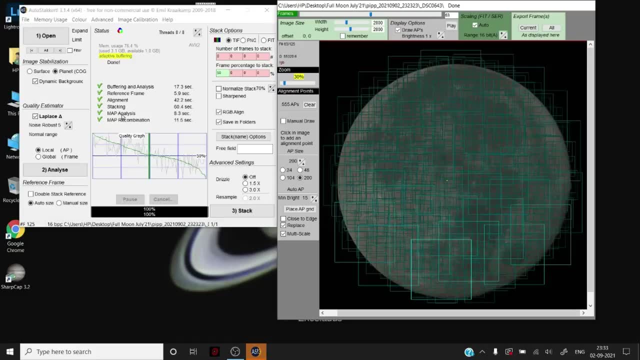 Once we are done with this and we are back, We are through the stacking process and our stacker. We have done all these steps. We have selected 50% of frames. basis The graph that it has showed us, though We knew the quality from the folder was good. 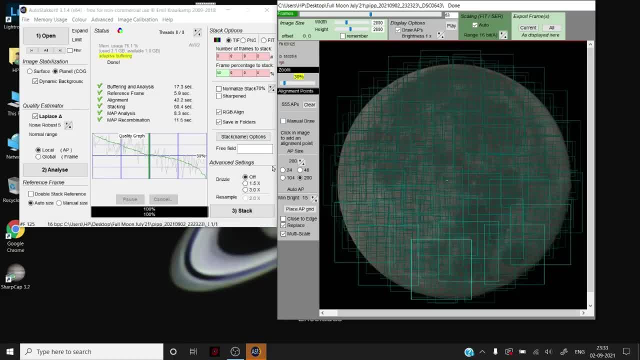 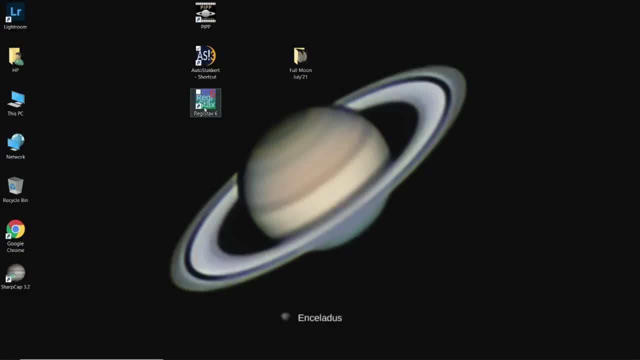 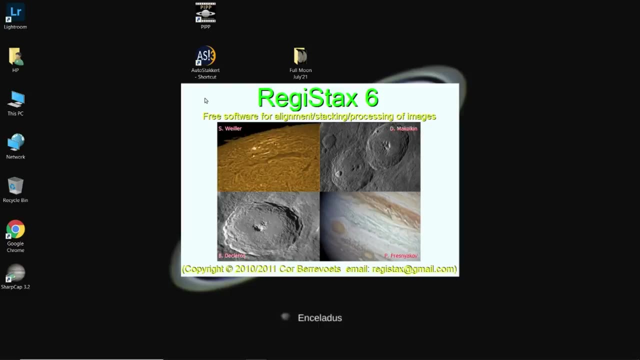 but that's not something which is bad. We have plenty of data to work with in register stacks, So let's close this And now let's jump into register stacks. This is where we are going to enhance the image that we have just derived by stacking. 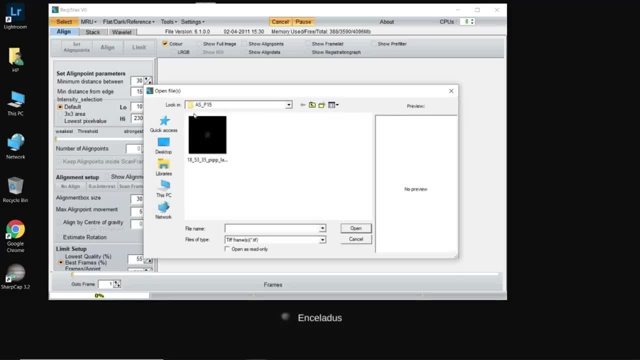 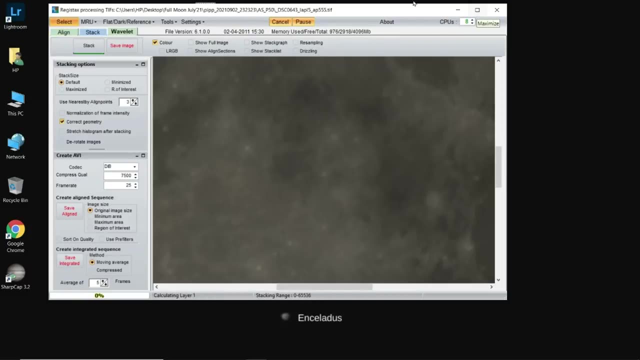 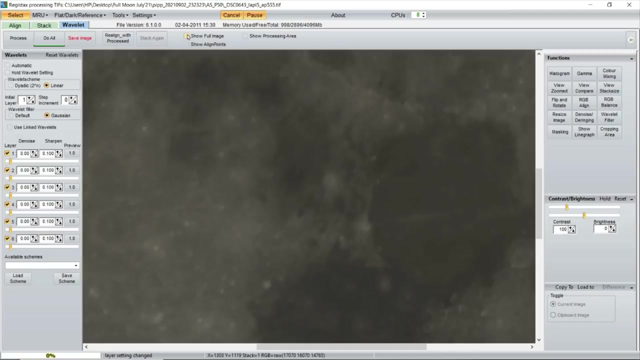 Let's open the folder on the desktop. This is our stacked image: 50% of 125 frames that we took off moon. Okay, So it's going to show us something Like this: You can always click on show the full image. 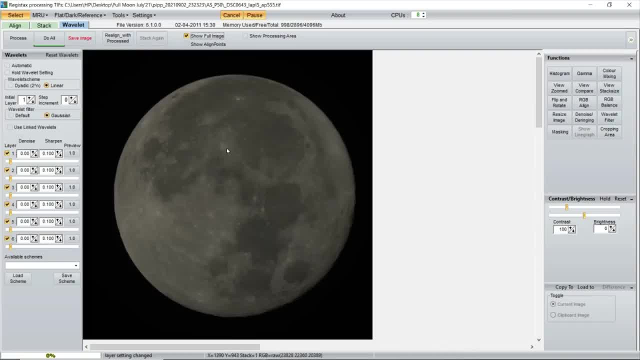 So now it's going to show you the full image Now, unlike planetary, we don't have to play much with your wavelets because we don't want over sharpening. If, in case, you do over sharpen, there is no way that you can remove it. 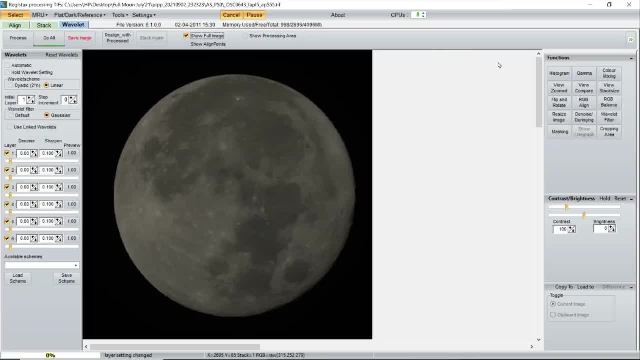 So again, be very careful when you play with the wavelets. Be very wary that once you have over sharpened your moon, there is no way that you know you could remove that in any other software. So I would advise you to go very gentle on this. 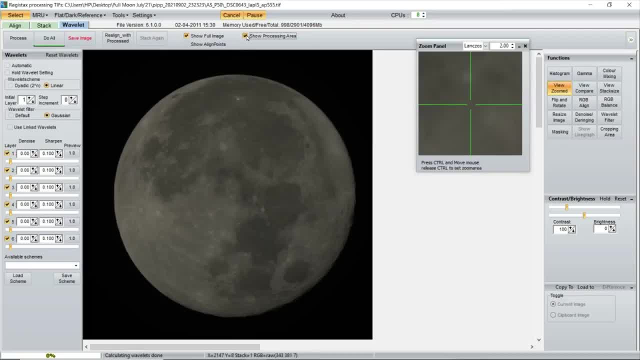 Now, this is the processing area, So I'm going to take care. It's going to show you the processing area. Where is that? I don't see those arrows somewhere. Okay, So we are going to do stepwise. First layer normally gives you a lot of. 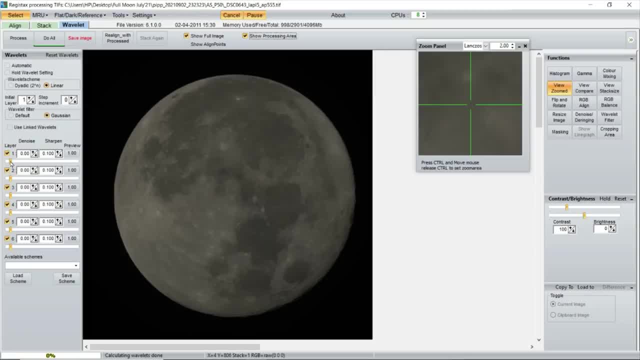 It gives you a lot of noise, but I somehow like to go with the first layer And if you see what I am doing, where is the processing? Look here in this zoomed image, And I think we are somewhere here. I normally like to keep the edges in focus because that's where. 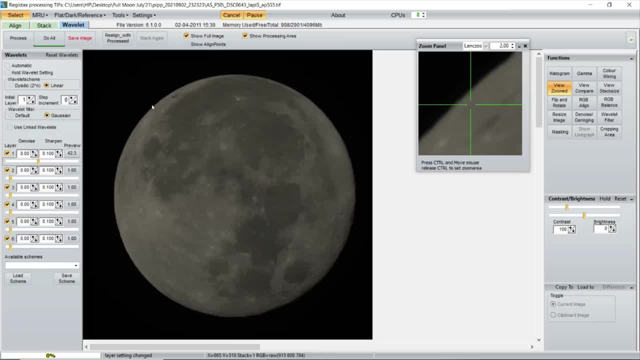 you know, if you've done over stacking, that's where the artifacts, would you know they would just show here first. Okay, So we are here and I'm going to sharpen very gently Just one And I'm going to do denoise because, yes, 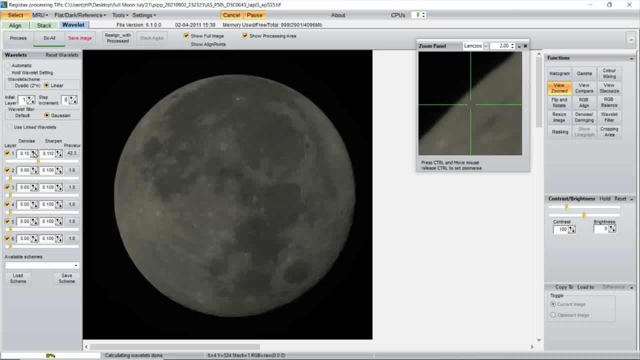 it does add a lot of noise to your image And DSLR images. you can't, you know, work more with the noise. So, again, being very careful, I would take this to up to, let's say, 20.. And I just like to play with the last layer. 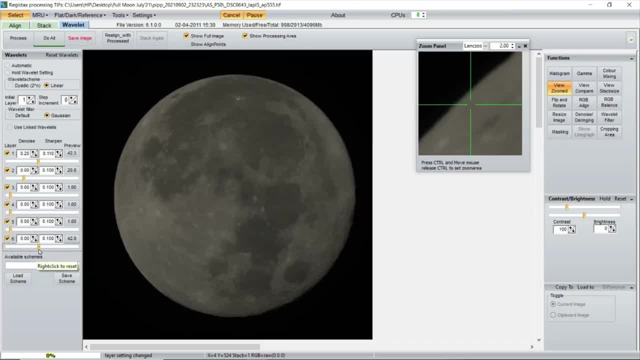 That's it. I don't do much, Okay. So this is where we are. We're going to do sharpening here and we're going to do some denoise. So you can't see the effect. You know, you can't see this what's happening here, because there's a little teeny tiny. 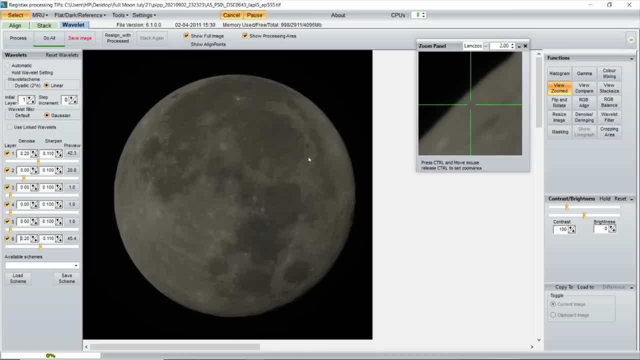 area of processing here. You can't see it right now. If I press, do all this is where you want to see what you've done on the wavelets. It's going to show here. You can see, slowly and gradually, The details are emerging, and look at the change. 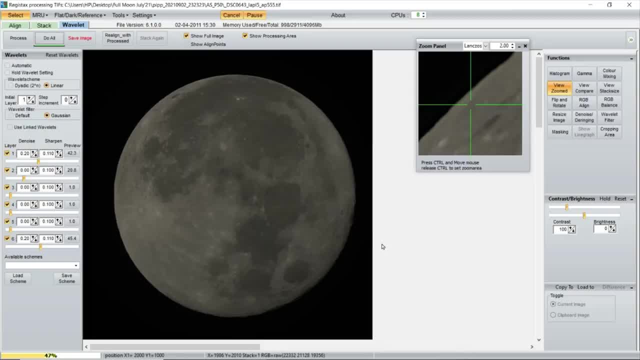 It has brought to your very dull image. It has a lot of data. It's a stack of 50% of 120 frames, So it has a lot of data. It's just that you need to enhance it, And by looking at this: 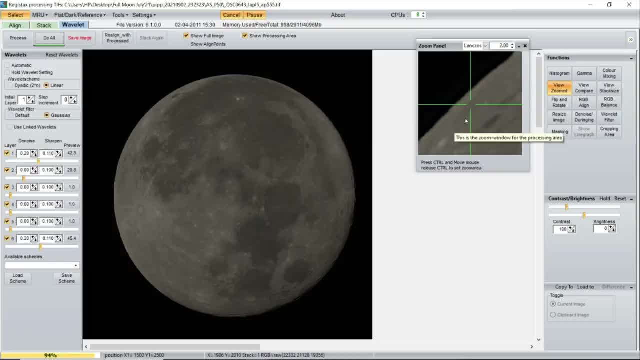 I don't think that I have over sharpened it anywhere. The edges are still very natural. There's no artifact here. I can check Right, So this looks fairly Okay. Look at the details here. Oh, my God, And this is through a DSLR, and you can see that there is no noise. 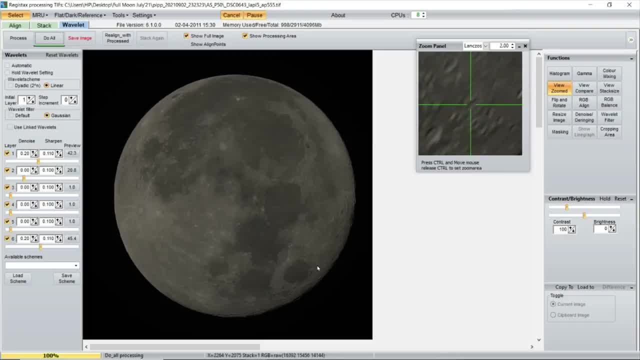 Okay, We have taken care of the noise. Okay, So this is look at the details. Oh, now we can still do a little bit more in terms of sharpening, because I don't see any artifacts emerging. I can still drag it. 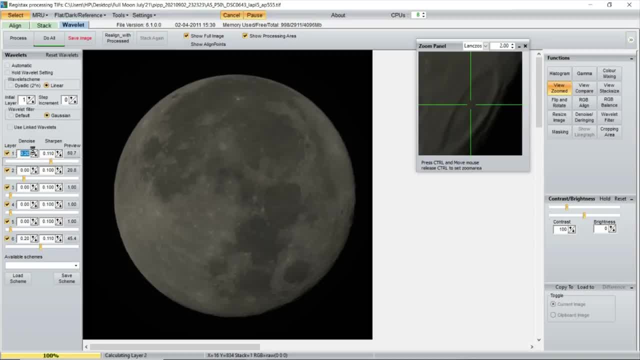 but this layer is definitely going to add noise. So just ensure that you denoise properly as you Increase the amount of sharpening. Just ensure that you do that And let's see, Let's see. What do we have here? This dual thing takes 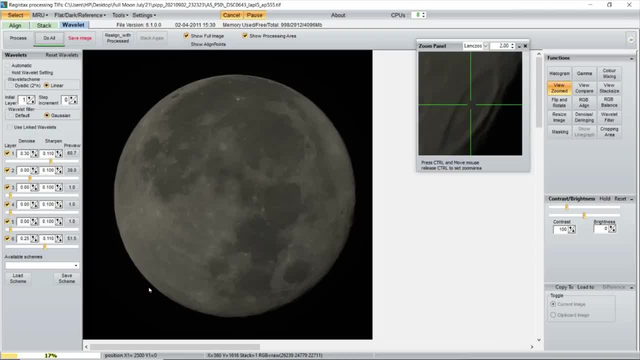 It takes a while because this is a large file and it's going to Go layer by layer And it's going to show you. Okay, I don't still see any kind of over sharpening. We are Doing quite well here. 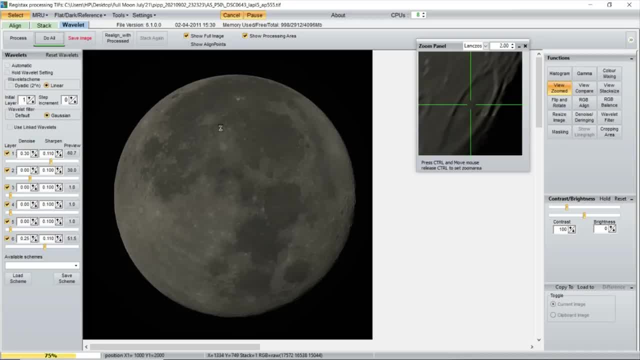 Oh lovely, This is looking nice. So I would Still recommend that we again do a bit of more sharpening. We can do this. The data is quite good. Okay, I see a bit of noise. Yeah, There's noise. 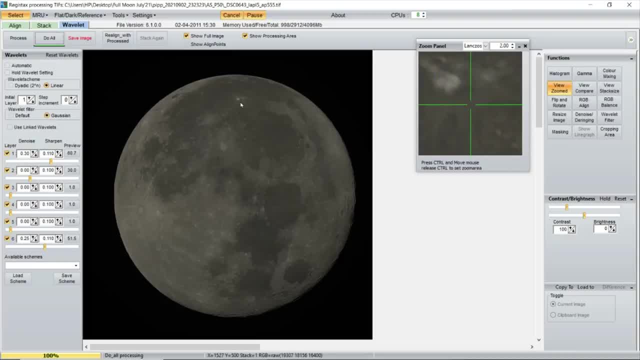 Yeah, So In that case, We are not going to play with The First Layer, We are going to work Our way To the second layer And I think, Yeah, We can do a bit of Denoise. 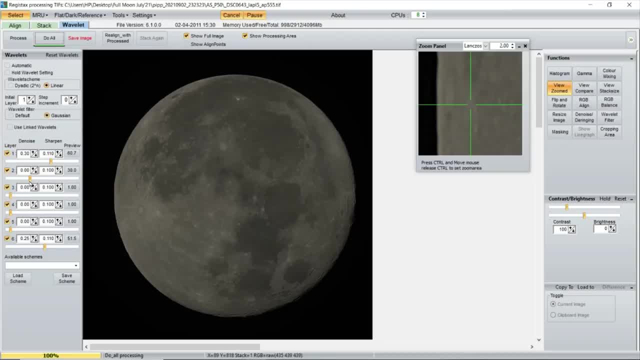 And I think, Yeah, We can Do A bit of Noise. Yeah, There's noise, Yeah, So We can do a bit of Denoise here, Because I see a little bit of noise emerging. Okay. 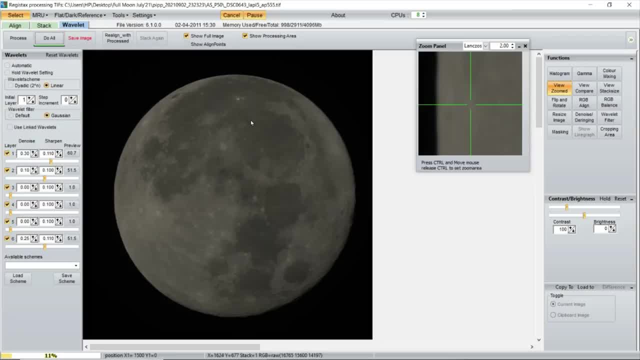 Let's see where we are. It's a tedious process. You need a lot of patience to work with wavelets, So Anything that you overdo It's going to impact your final image. So Just be patient, Just check. 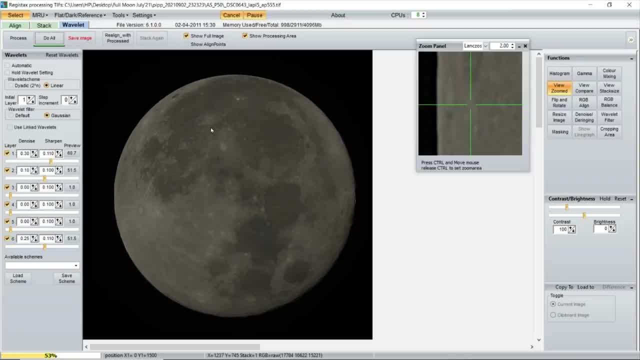 Every time Press do all, And it's I'm. I know that it's taking a while, But It's all worth it. It is definitely worth it. It enhances your image. It does not give you any artifacts And 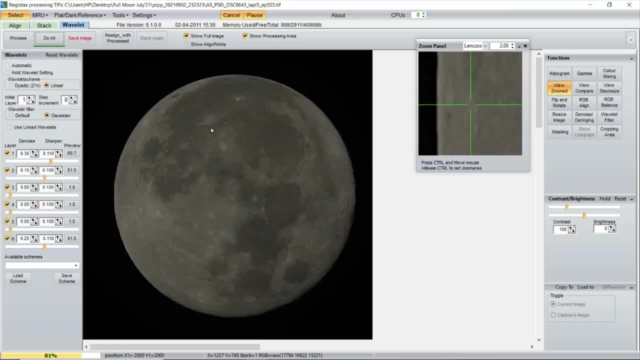 What more do you want? A good image, Right, So Let's work towards it, And I think I am quite happy with this. If I look at the edges, Yep, They are sharp, They are not overdone. 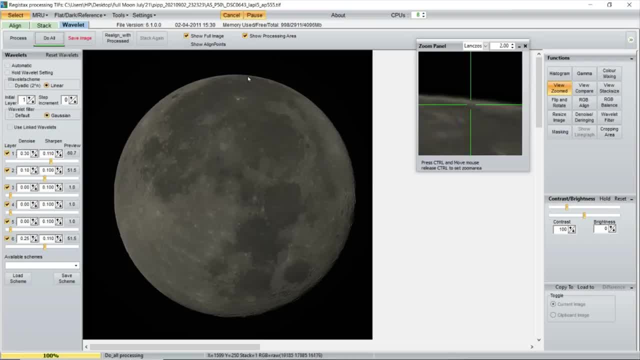 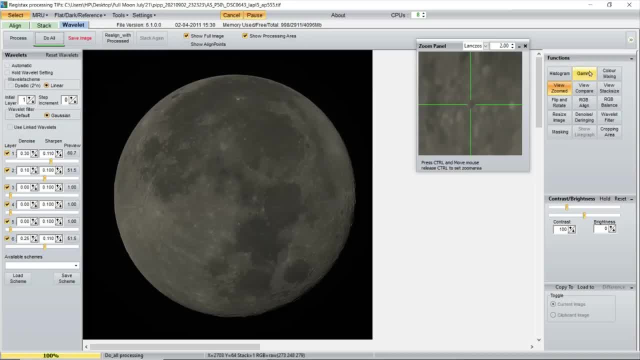 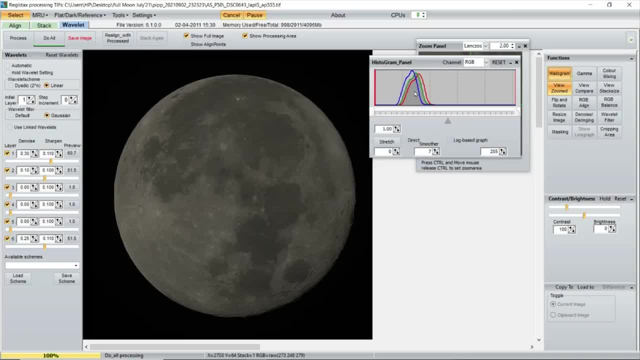 We don't want to create anything Which looks very unnatural. We can look at the histogram. It's quite a line. As I said, When you look at your histogram In your DSLR While you're shooting, You're taking test images. 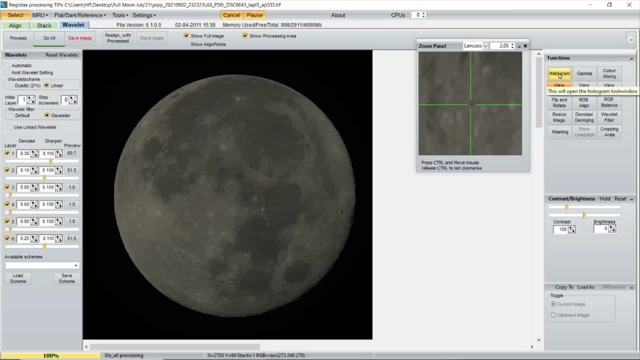 You need you check histogram while you're imaging through dslr. we can do rgb balance in this, though we can do this in photoshop. we can do it in other softwares. you can do auto balance here. it's just going to look like a grayscale image. so this is. 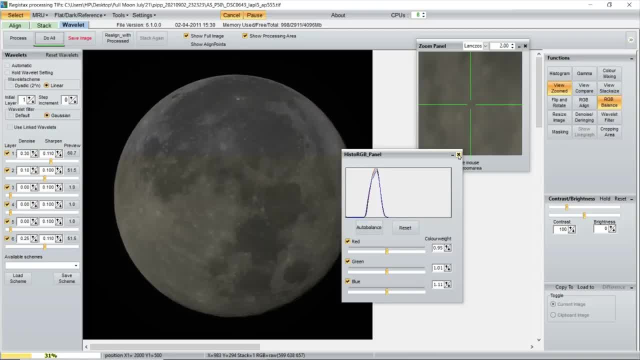 something which is your choice, completely your choice. i leave it to your taste. if you want to do this, you can, and this is going to be your final image. this is how it looks, how you know how big a difference it makes once you've stacked your images and 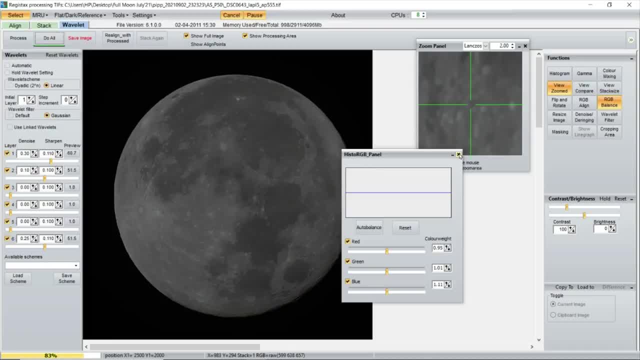 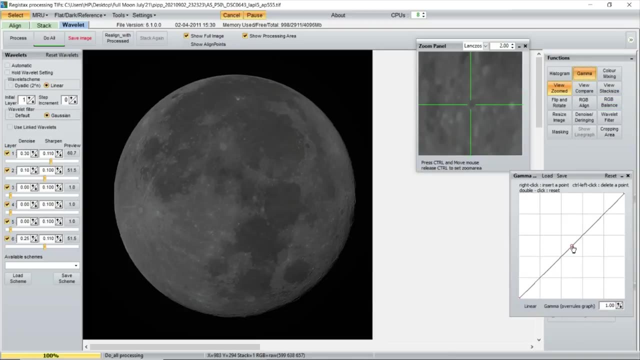 another thing that i would recommend in this to do is just to check your gamma. you can increase the brightness because moon- full moon- is especially very bright. so let's look at the gamma, let's see if we increase. so this is the processing area. you know, this is this teeny bit of. 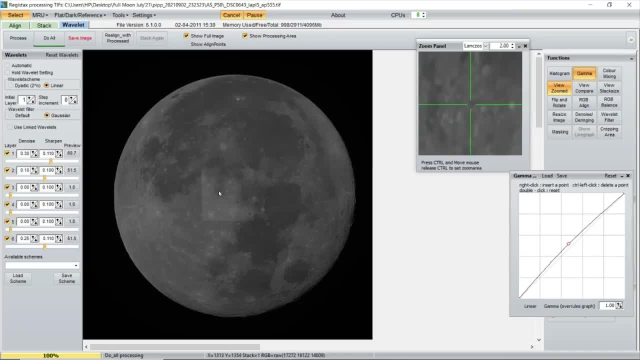 the center part of the moon is the processing area. this is where all the processing is taking place and i think i like this a bit better. but i can increase a bit of brightness. you can do this while you're you know processing your standard it in some other software, but i like to work everything in register so that i have very 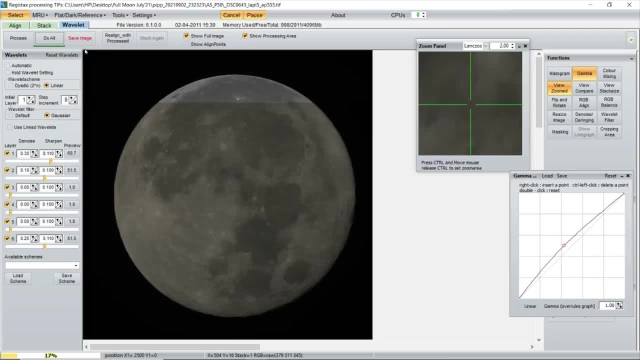 minimal amount of work to do. now look at the transformation. it is just happening right in front of your eyes. this is how your moon is going to appear, and this is full moon, full, bright moon. and you've just increased the iso and you've increased the shutter speed, and this is the 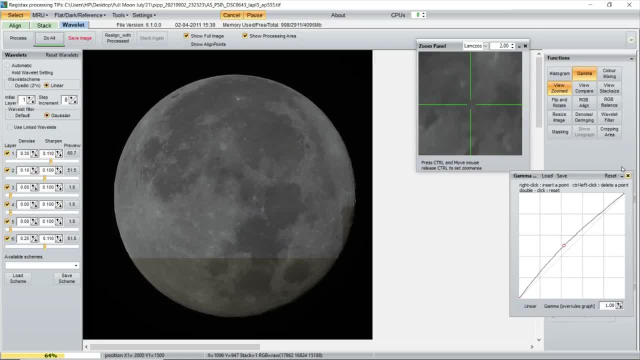 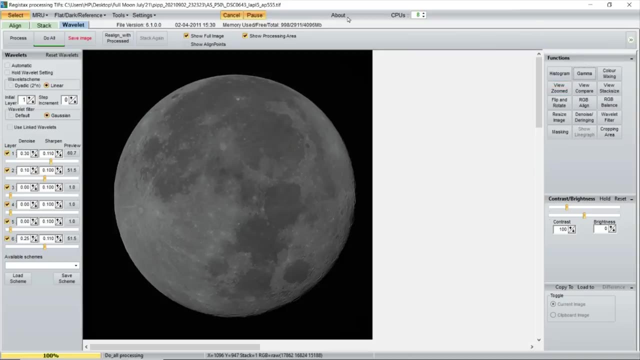 image that you get. i'm quite happy with it. this is something which is as for my taste and um, let's close this. we are done, okay, cool. so this is the final image. we're going to save this in the folder. it's automatically going there. it's not going to go anywhere. this is 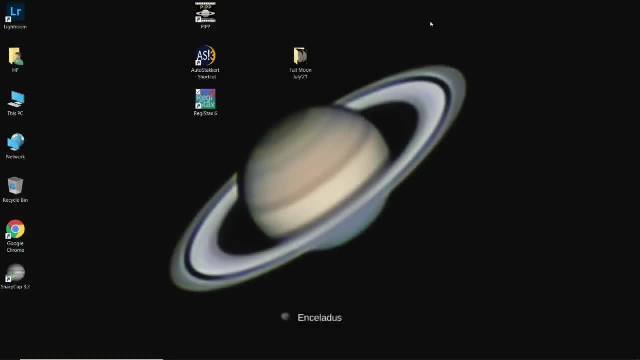 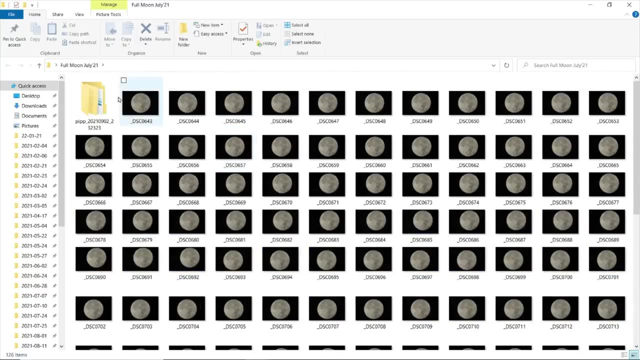 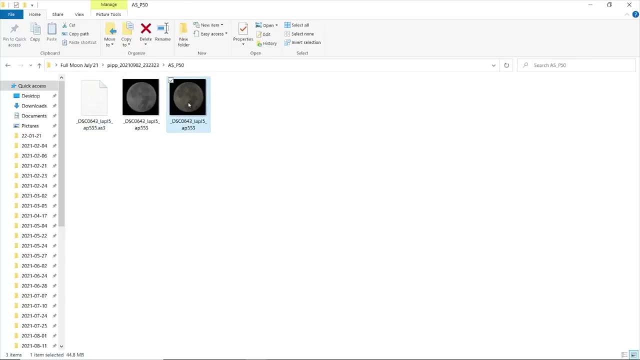 what i have learned this year. this was very new to me. i'm quite happy that i was able to not only take images through dslr and my telescope, but i could process through pip. i could use some of the planetary tricks that i've learned. this is the outcome of your 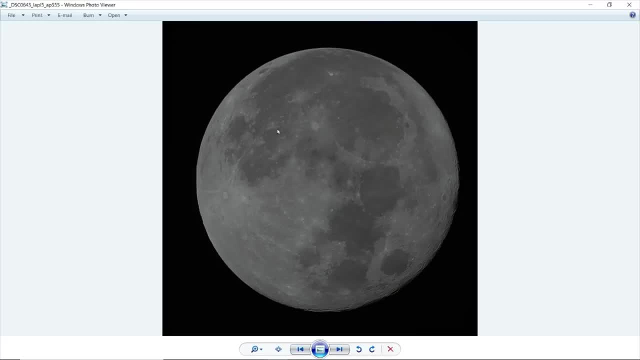 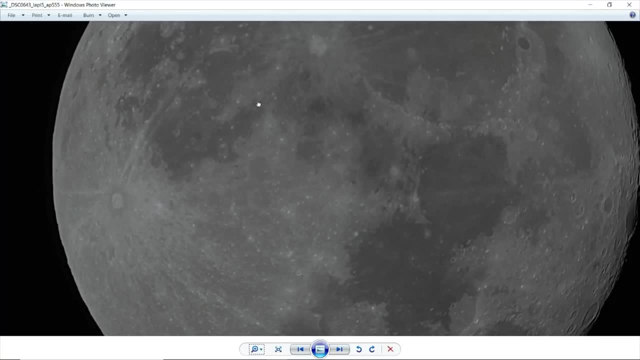 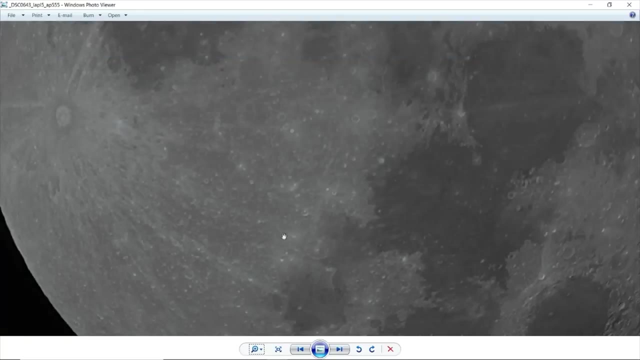 order stackered and this is how it looks in your uh register image. the the image. if i you know, i choose to show you a closer. look at this. look at this. i mean, this is something very, very beautiful, very pretty, very detailed image of moon. you can. 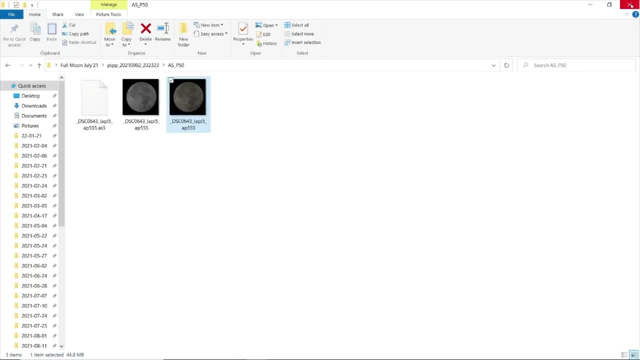 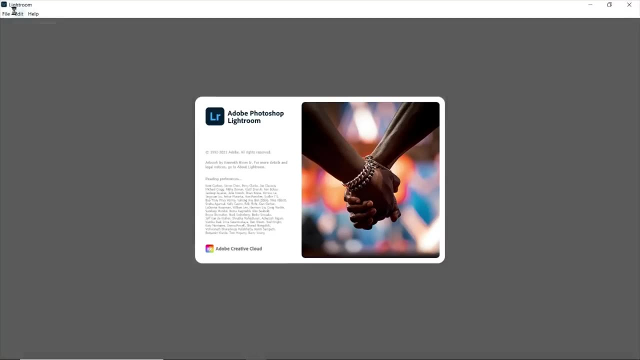 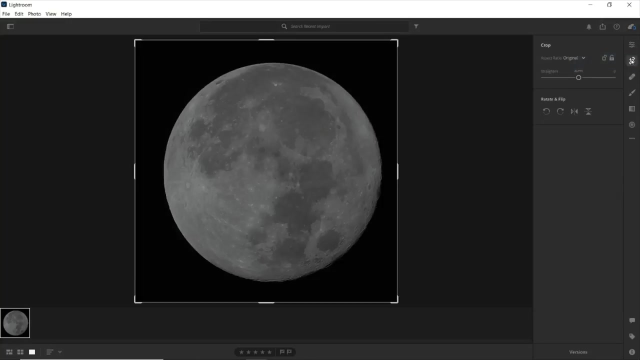 now choose to take it to any software of your choice. you can. i mean, i can- show you a bit of lightroom. mineral moon is a different process. i will need another tutorial for that. now you can find much more detail about the estuvim starve. it will ensure that you have complete rodeo. 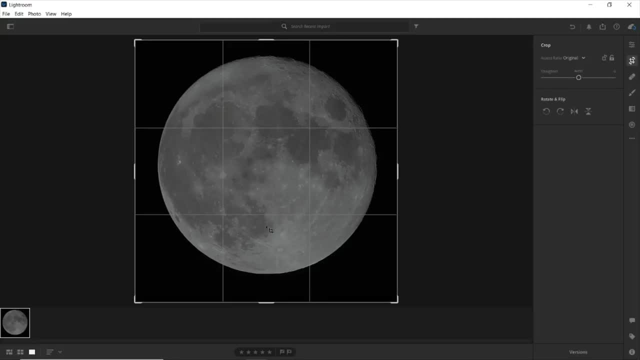 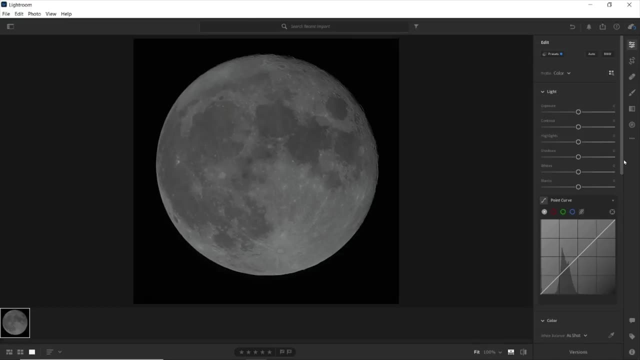 click the link that i shared with you to see the changes that i mentioned to the third rule. the triangle crater is looking somehow like a beautiful, completely different image, mental and underneath that. i just wanted to once again show you this. you could definitely edited to go physically so cool. so what i'm going to do is just completely change my ным. 1, if and when every. 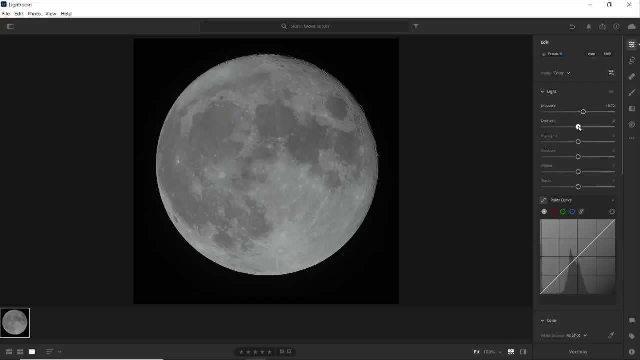 sake, is going to become public in my project because and then it's going to change into my nm1- and a bit of exposure contrasting- yes, it does enhance it is, you know- add a bit of highlight, shadow, decrease a bit. we're gonna increase on the whites and black. 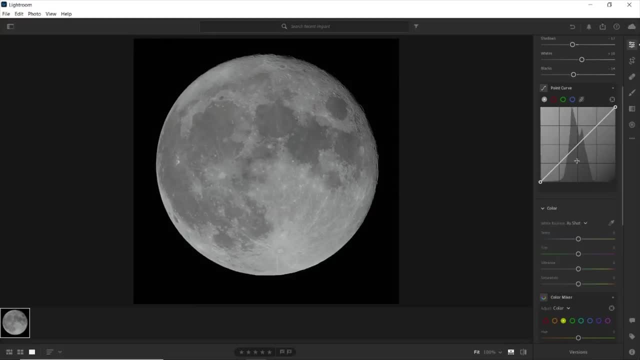 will decrease. so this is what you can do. you can further work into colors. I normally kind of play around with this section a bit. you can create colors. you can see the mineral colors appearing. I mean, this is a very rough way of creating a mineral moon. this is not a complete process, I'm just showing you. 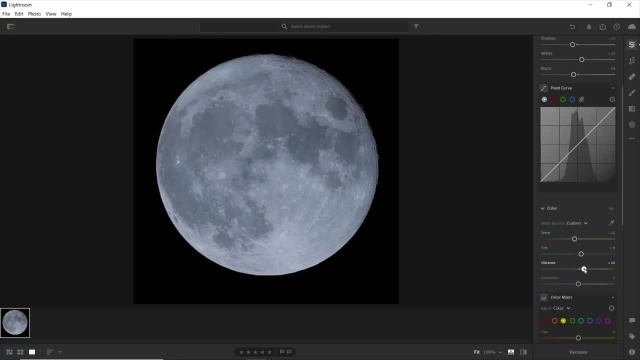 what you can do with your Registax image. you can add a bit of vibrance and once you add saturation, you're going to see that you getting a bit of a lot of blue color. you can add a bit of tint here, and this is something you know you. this is completely your personal taste. this is 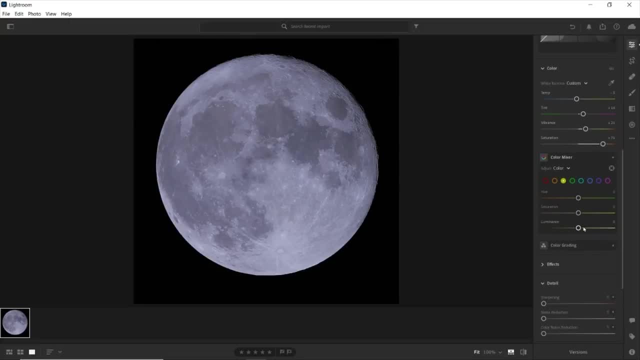 what I like. this is how I like to see the final results of my image. you can do sharpening here as well and do a bit of noise reduction. you can do sharpening here as well and do a bit of noise reduction. so this is what you know. there's so many things that you can do once you have. 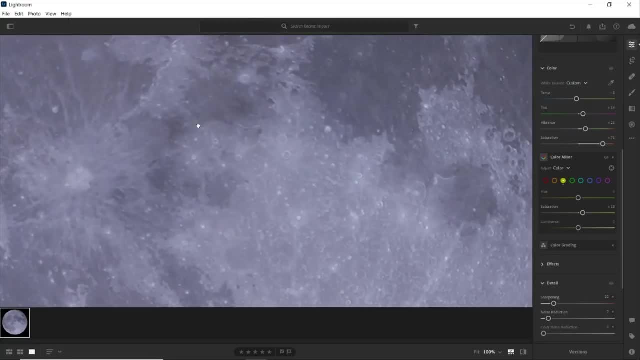 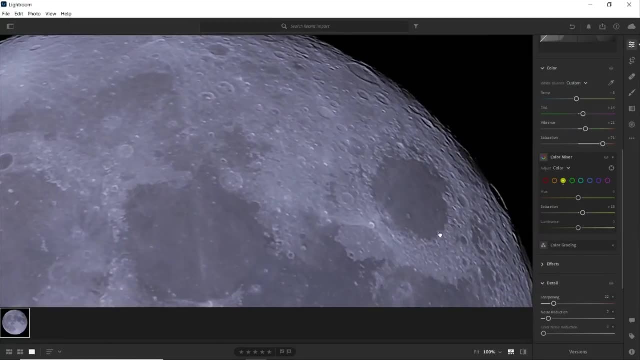 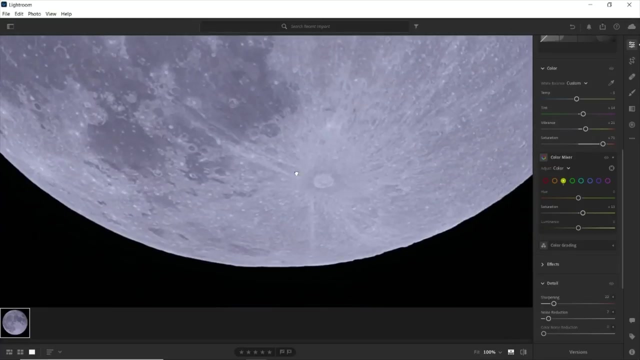 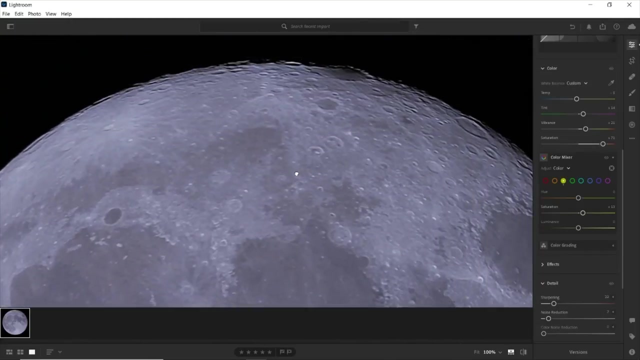 processed a wonderful full moon image. you see, it is noise free. the sharpening is completely precise. look at the depth that you have derived out of a DSLR image and you can create a wonderful mineral moon. this is the foundation of creating a mineral moon. it is very clear, very precise. I mean completely a very